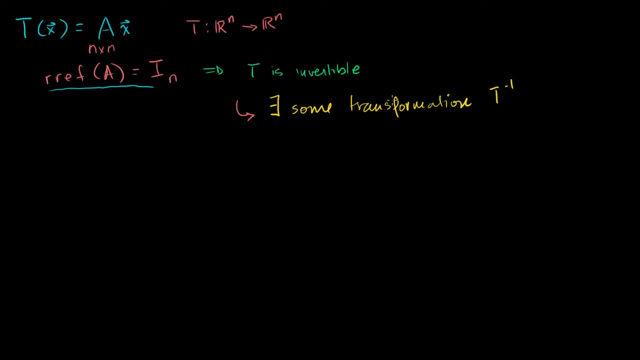 inverse, T inverse like that, or T to the minus 1, such that the composition of T inverse with T is equal to the identity transformation on your domain, The identity transformation, The identity transformation on your domain, And the composition of T with T inverse is equal to the. 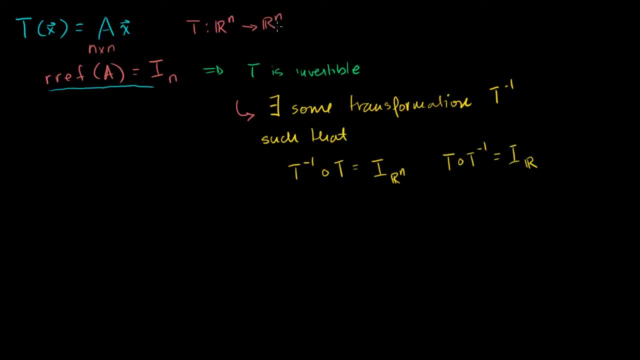 identity transformation on your codomain, Just like that. And just to remind you what this looks like, let's draw our domains and codomain. Our domain is Rn And our codomain is also Rn. It's just like that. 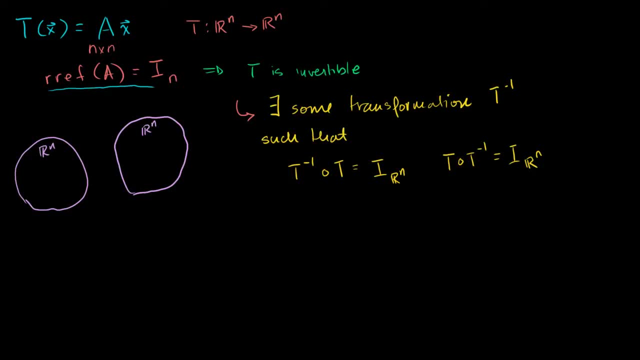 Codomain is also Rn, So if you take some, If you take some vector in your domain, apply the transformation T, you're going to go into your codomain, so that is T. And then if you apply the T inverse after that you're. 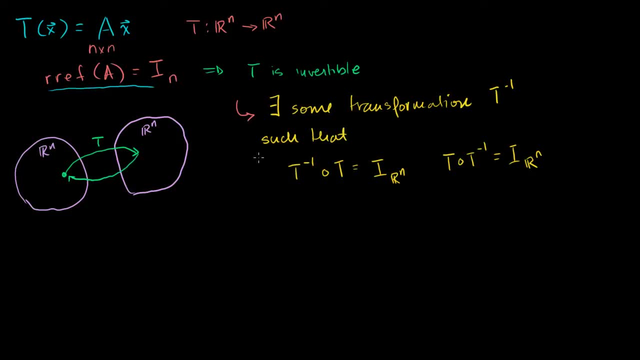 going to go back to that original X. So this says: look, you apply T and then you apply T inverse, You're just going to get back to where you started. It's equivalent to the identity transformation. It's equivalent to the identity. 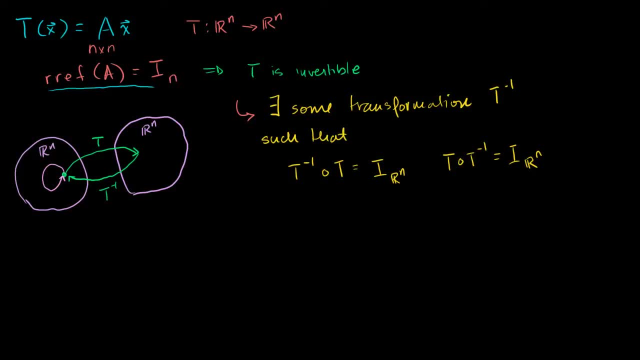 transformation, just like that. This is saying: if you start here in your codomain, you apply your inverse first, You apply this inverse transformation first, Then you apply your transformation. You're going to go back to the same point in your codomain. 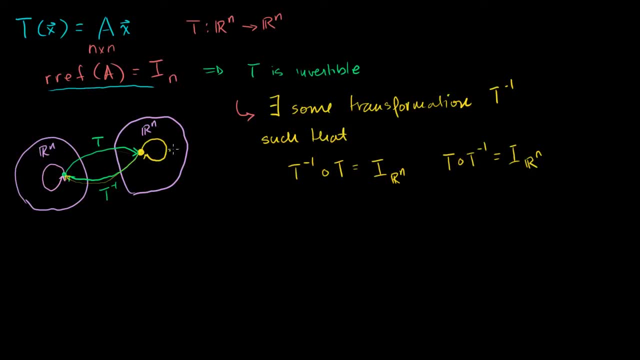 So it's equivalent to the identity transformation in your codomain. It just happens to be, in this case, that the domain and the codomain are the same set: Rn. Now we know what a transformation, what it means to be invertible. 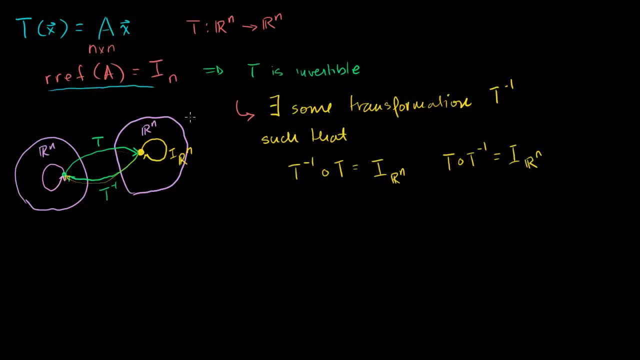 We know what the conditions are for invertibility. So this begs. the next question Is this: We know that this guy is a linear transformation. In fact, that's one of the conditions to be able to represent it as a matrix, Or any transformation that can be represented as a matrix. 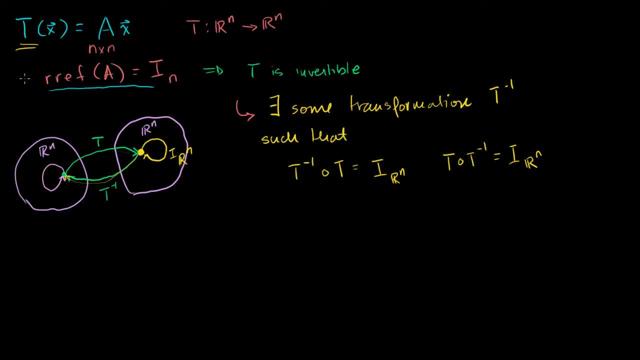 vector product is a linear transformation. So this guy is a linear transformation. But the question is: is T inverse a linear transformation? Now let's review what the two conditions are that we need to have to be a linear transformation. So we know T is a linear transformation. 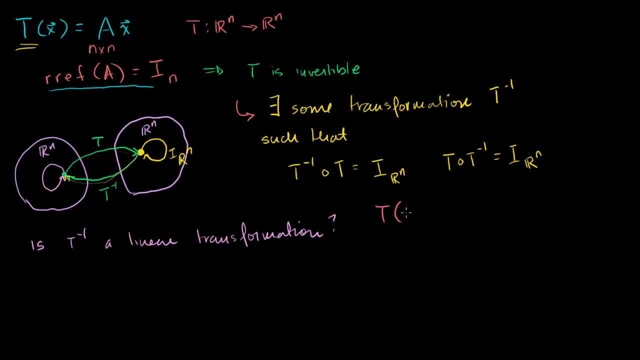 So we know that if you apply the transformation T to two vectors, let's say x and y, if we apply it to the sum of those two vectors, it is equal to the transformation of the first vector plus the transformation of the second vector. 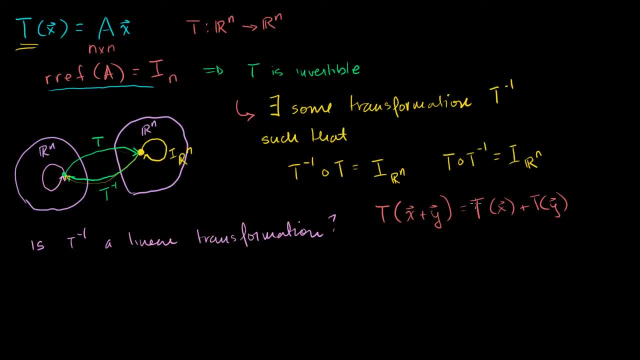 That's one of the conditions, or one thing that we know is true for all linear transformations. And the second thing that we know is true for all linear transformations is if we take the transformation of some scaled version of a vector in our domain, it is equal to the. 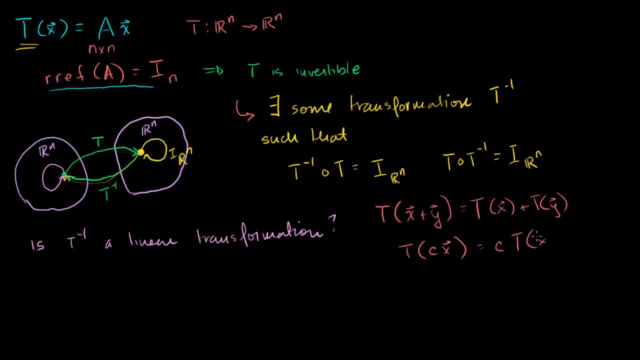 scaling factor times the transformation of the vector itself. These are both conditions for linear transformations. So let's see if we can prove that both of these conditions hold for T inverse, for this guy right here. So to do this, let's just apply, let's do this little. 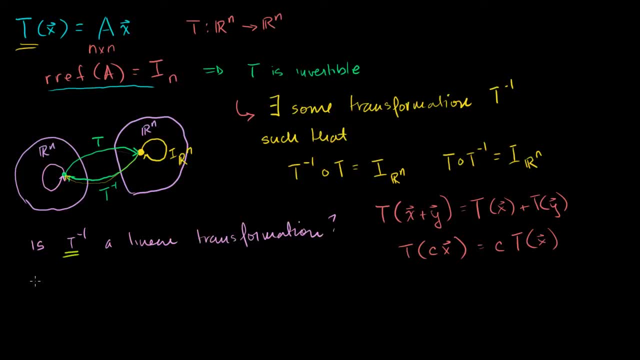 exercise right here. Let's apply T. let's take the composition of T with T inverse of two vectors, A plus B. Remember, T inverse is a mapping from your co-domain to your domain, although they're both going to be Rn in this. 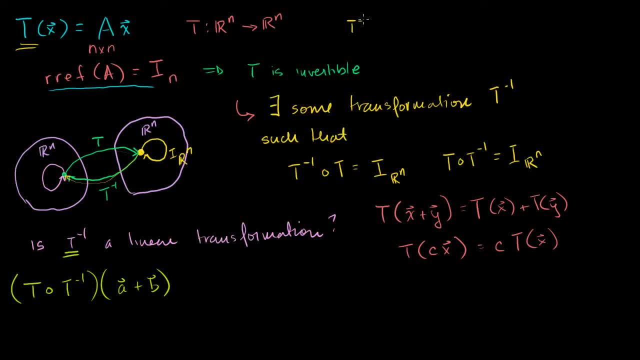 case, but T inverse maps from this set to that set. Let's just write it up here: T inverse is a mapping from your co-domain to your domain, although it looks identical just like that. OK, So what is this going to be equal to? 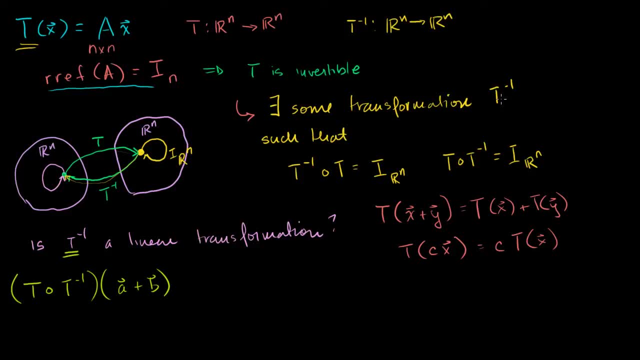 Well, we just said, by definition of your inverse transformation, this is going to be equal to the identity transformation on your co-domain. So, assuming that these guys are members of your co-domain- in this case Rn- this is just going to be equal to A plus B. 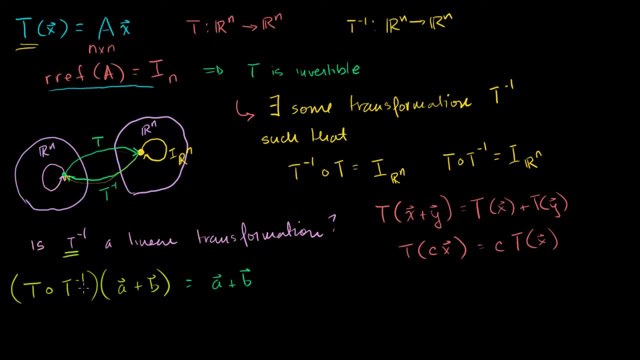 This thing, the composition of T with its inverse, by definition, is just the identity transformation on your co-domain. So this is just Whatever I put in here. If I put in an x here, this would be an x. If I put in an apple here, this would be an apple. 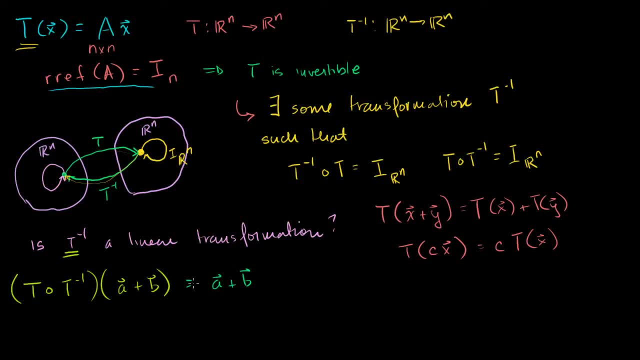 It's going to be the identity transformation. Now, what is this equal to? Well, I could use the same argument to say that this right here is equal to the identity transformation applied to A. And I'm not writing the identity transformation, I'm writing this. 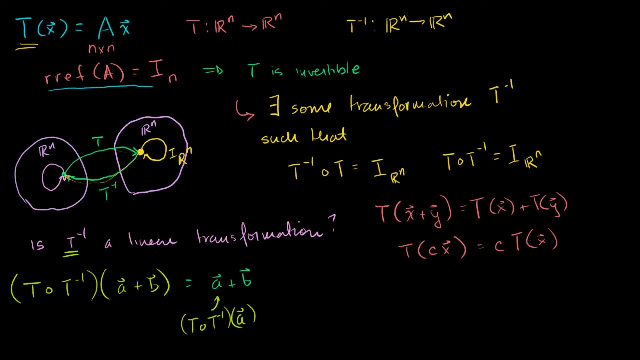 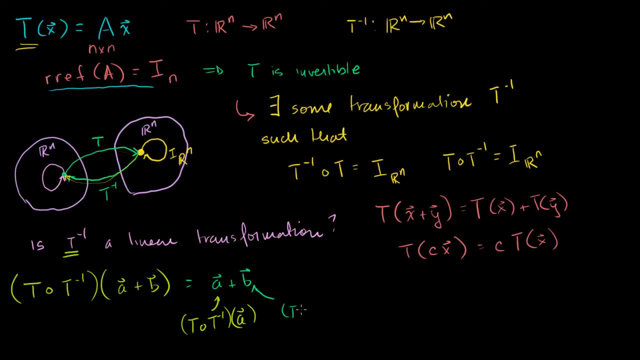 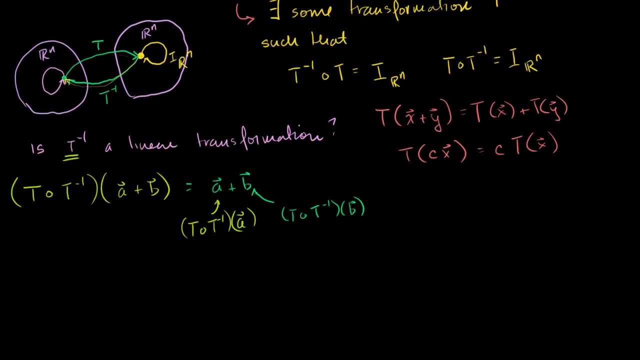 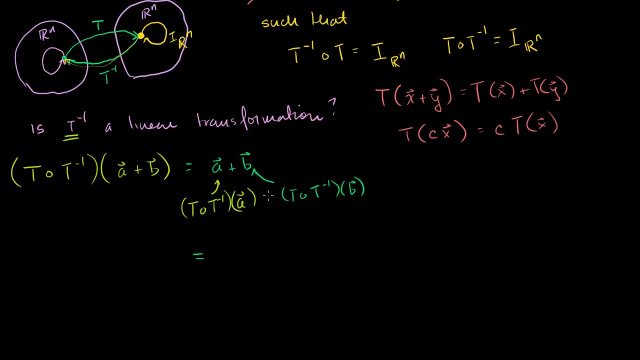 composition of T with T inverse applied to B. So we can rewrite this thing right here as being equal to the sum of these two things. In fact we don't even have to rewrite it, We can just write it's equal to. This transformation is equal to the sum of these two things. 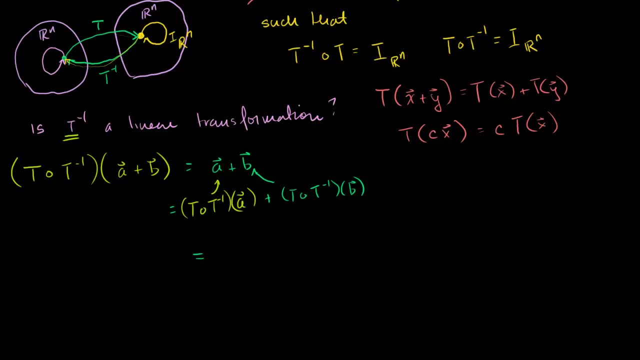 This transformation is equal to this And maybe an easier way for you to, I guess, process it is, we could write this as: T of the T inverse of A plus B is equal to T of the T inverse of A plus T of the T inverse of B. 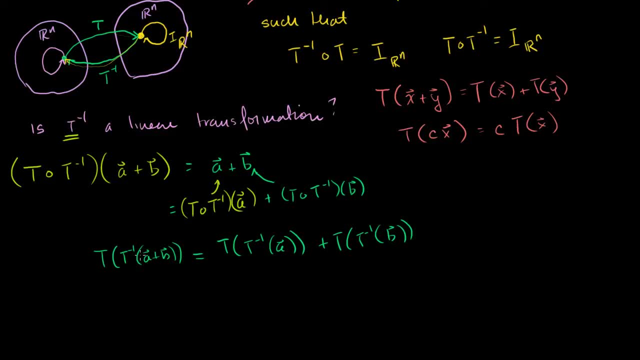 And this, should you know. I don't know which one your brain processes easier, But either of these. when you take the composition of T with T inverse, you're just going to be left with A plus B. When you take the composition of T with T inverse, you're. 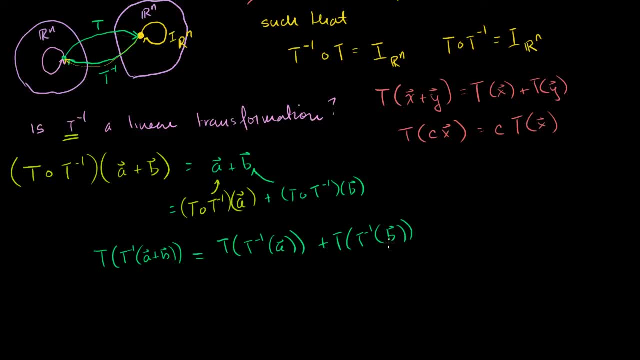 left with an A. When you take the composition of T with T inverse, you're just left with a B there. So in either case you get A plus B. When you evaluate either side of this expression, you'll get the vector A plus the vector B. 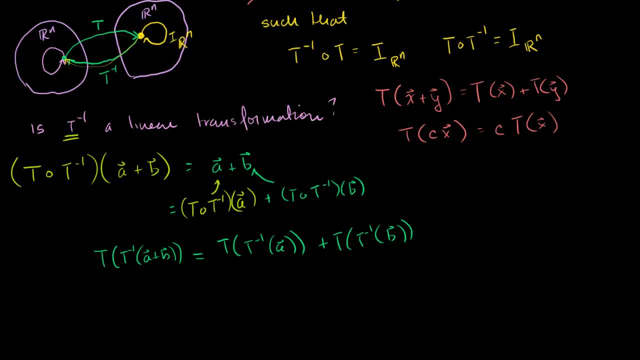 Now what can we do? We know that T itself is a linear transformation And since T is a linear of transformation, we know that t applied to the sum of two vectors is equal to t applied to each of those vectors. and, summed up, 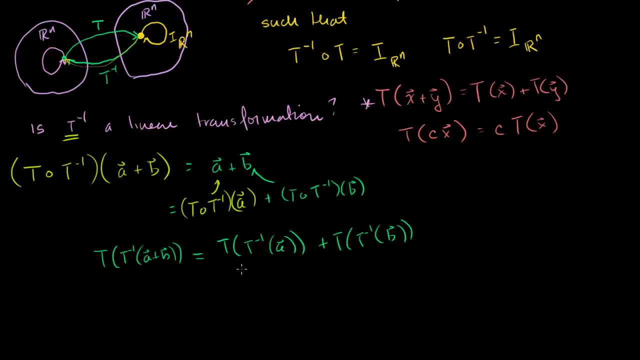 Or we could take it the other way: t applied to two separate vectors, so that we could call this one vector right here and this vector right here. So in this case I have a t applied to one vector and I'm summing it to a t applied to another vector. 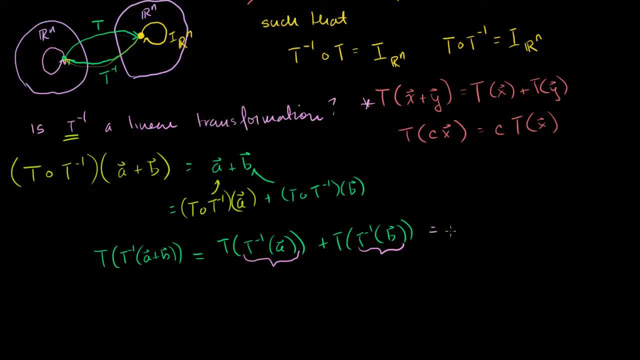 So it's this right here which we know is equal to t applied to the sum of those two vectors. So this is t applied to the vector t inverse of a. Let me write it here. So this is going to be equal to t inverse of a plus t. 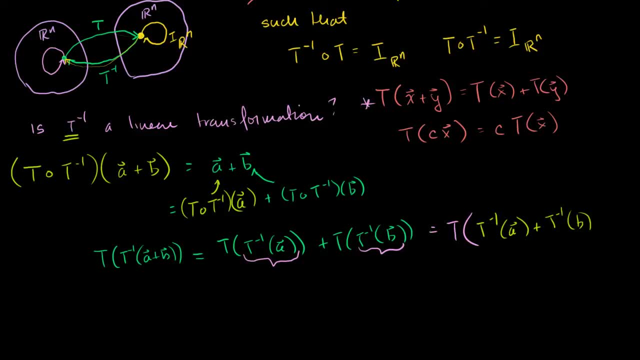 inverse of b. It might look a little convoluted, but all I'm saying is: look, this looks just like this. If you say that x is equal to t, then you're going to get. t is equal to t. inverse of a. 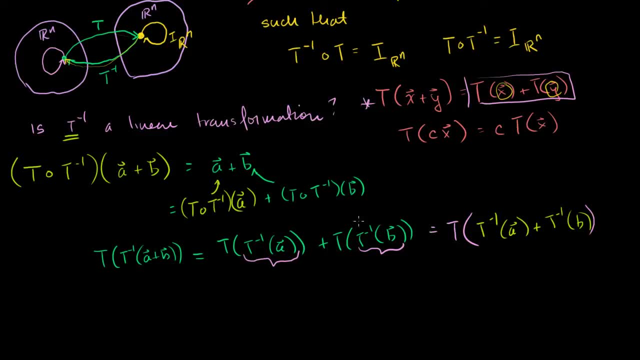 And if you say that y is equal to t inverse of b. So if this looks just like that, it's going to be equal to the transformation t applied to the sum of those two vectors. So it's going to be equal to the transformation t applied. 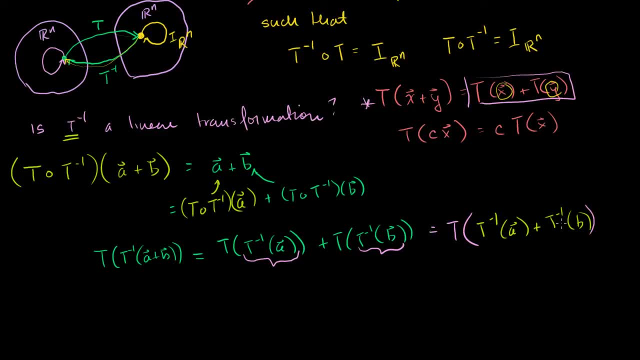 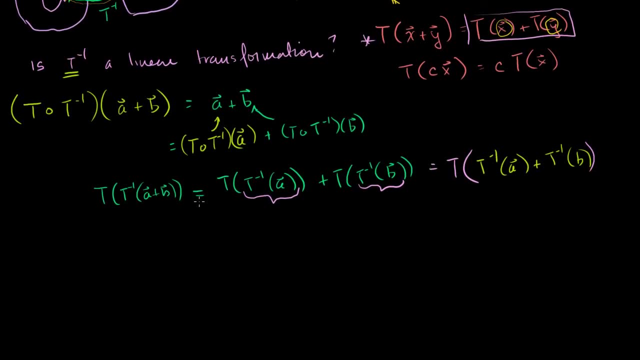 to the inverse of a, t inverse of a plus t inverse of b. I just used the fact that t is linear to get here. Now, what can I do? Let me simplify everything that I've written right here. So I now have. let me rewrite this. 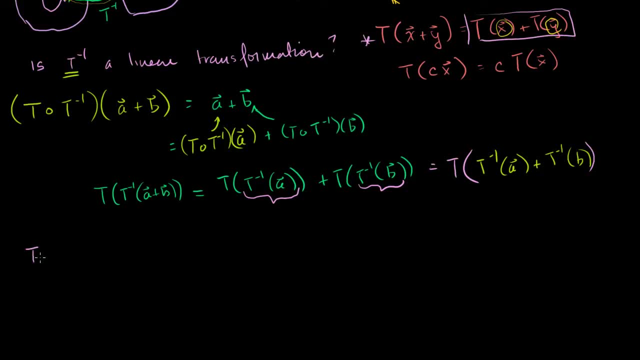 This thing up here, Which is the same thing as this: The composition of t with t inverse applied to a plus b is equal to the composition, or actually not the composition, just t applied to two vectors: t inverse of a plus t inverse of vector b. 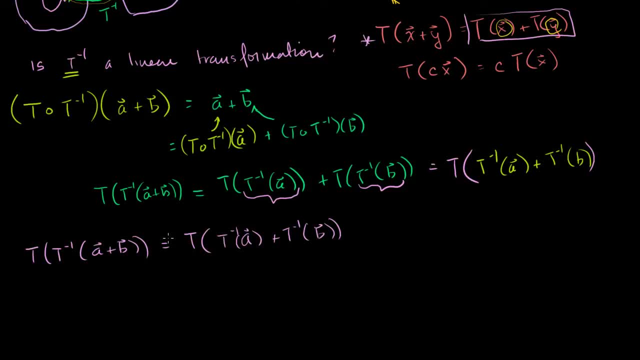 That's what we've gotten so far. Now we're very close to proving That this condition is true for t inverse, If we can just get rid of these t's, Well, the best way to get rid of those t's is to take the. 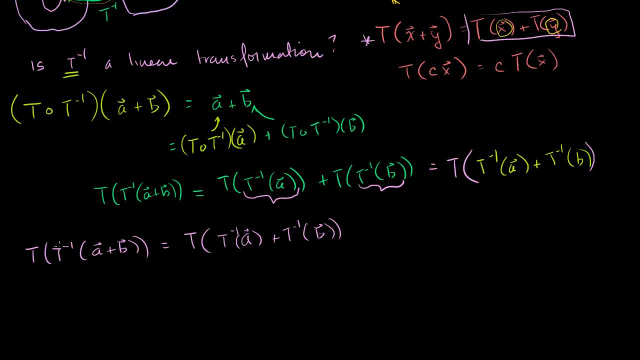 composition with t inverse on both sides. Or take the t inverse transformation of both sides of this equation. So let's do that. So let's take t inverse of this side. t inverse of that side should be equal to t inverse of this side. 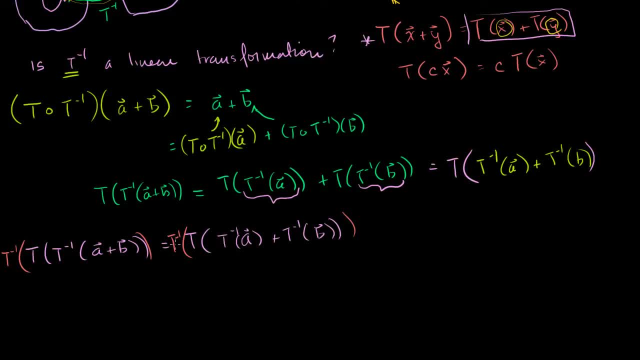 Because these two things are the same thing. So if you put the same thing into a function, you should get the same value on both sides. So what is this thing on the left-hand side? What is this? This is the composition of t inverse with t. that part. 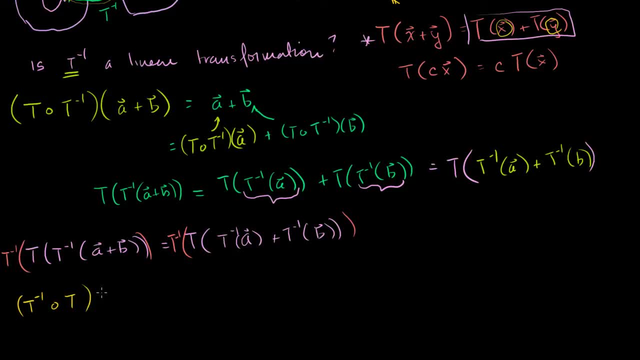 applied to this thing. right here, I'm just changing the associativity of this: Applied to t inverse of the vector a plus the vector b. That's what this left-hand side is, This part right here: t inverse of t of this. I'm just 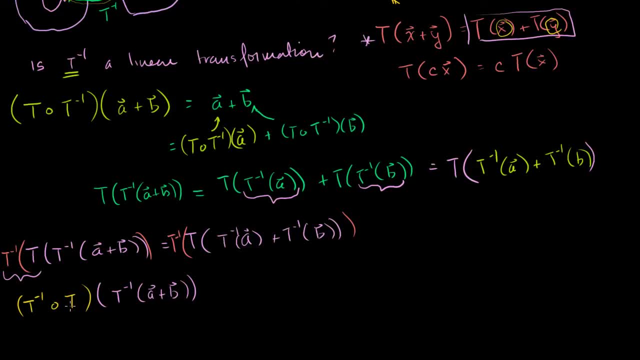 this first two steps I'm just writing as the composition of t inverse with t applied to this right here. That right there is the same thing as that right there. So that was another way to write that, And so that is going to be equal to the composition of t. 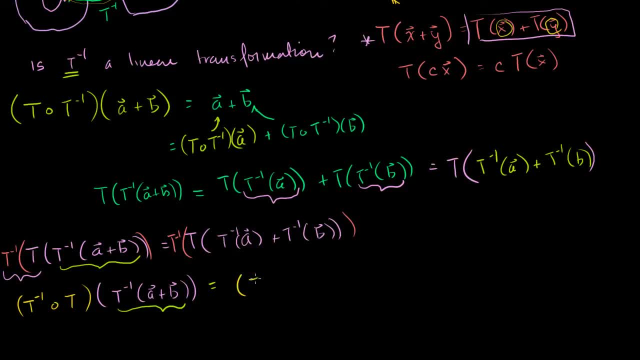 inverse with t. so I'll write it in the same color. The composition of t inverse with t, that's this part right here which is very similar to that part right there of t inverse of a plus t inverse of the vector b. 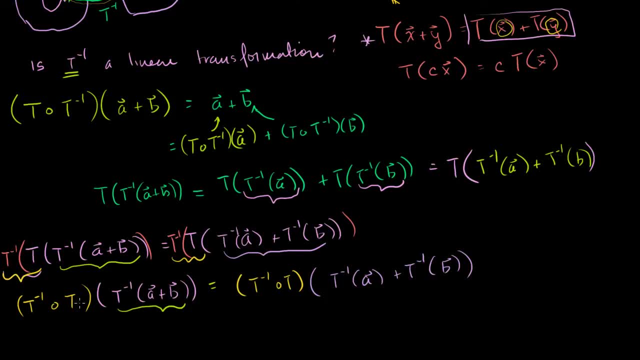 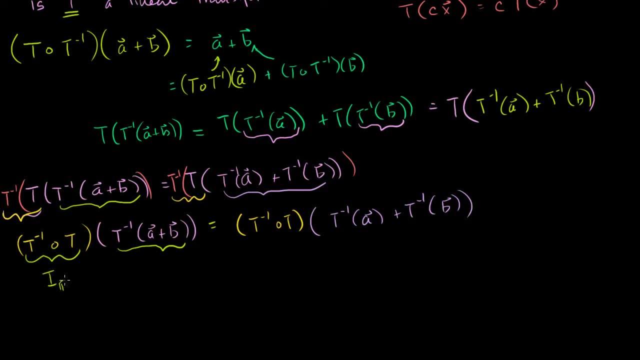 Now, by definition of what t inverse is. what is this? This is the identity transformation on our domain. This is the identity transformation on Rn. This is also the identity transformation on Rn. So if you apply the identity transformation to anything, 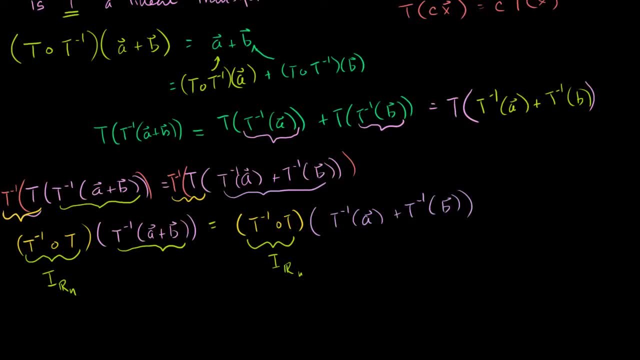 you're just going to get anything. So this is going to be equal to- and I'll do it on both sides of the equation. this whole expression on the left hand side is just going to simplify to the t inverse of the vectors a plus the vector b. 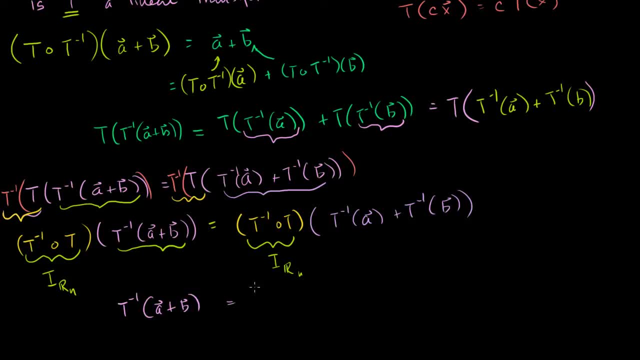 And the right hand side is just going to simplify to. this thing is equal to, because this is just the identity transformation. so it's just equal to this one: t inverse of the vector a plus t inverse of the vector b, And just like that we've met t inverse. 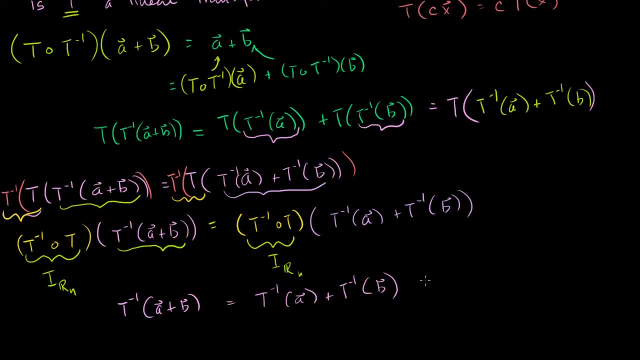 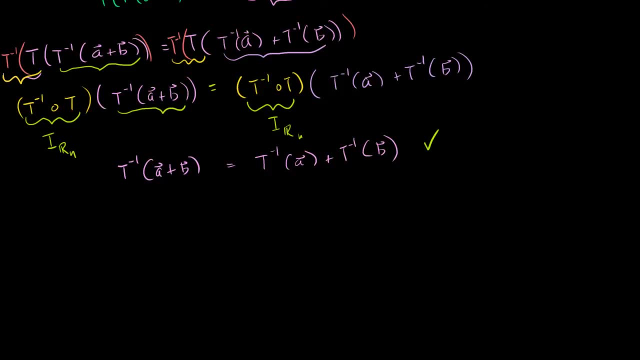 This has met its first condition for being a linear transformation. It's met its first condition. Now let's see if we can do the second condition. Let's take t of. let's do the same type of thing. Let's take the composition of t with t inverse of. let's take 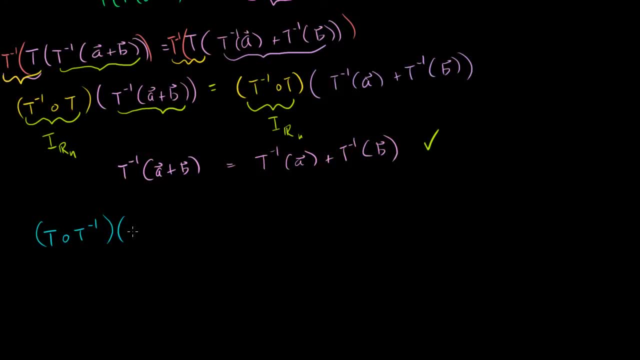 the composition of that on some vector. let's call it ca, just like that. Well, we know what this is equal to. This is equal to the identity transformation on Rn, So this is just going to be equal to ca. 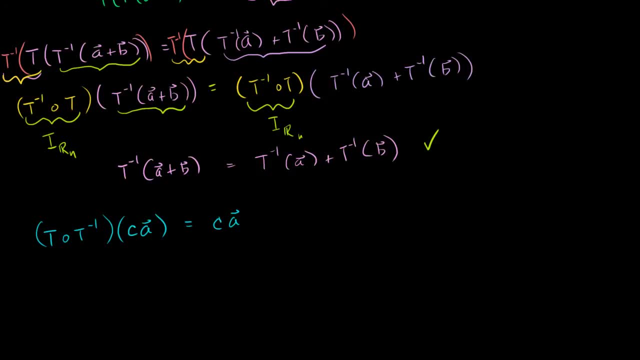 Now, what is a equal to? What is this thing right there equal to? I'll write it on the side right here. Let me do it in an appropriate color. We could say that a, the vector a, is equal to the transformation t with the composition of t with t. 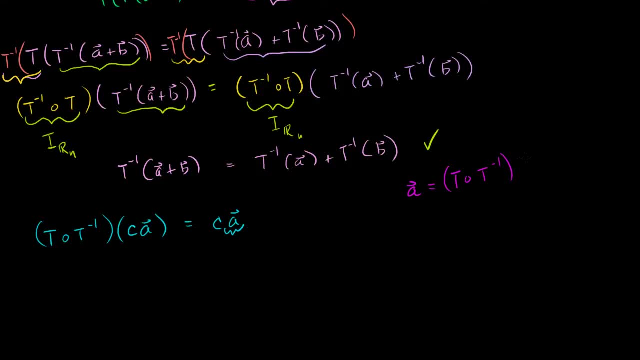 inverse. t inverse Applied to the vector a, because this is just the identity transformation, So we can rewrite this expression here as being equal to c times the composition of t, with t inverse applied to my vector a, And maybe it might be nice to rewrite it in this form instead. 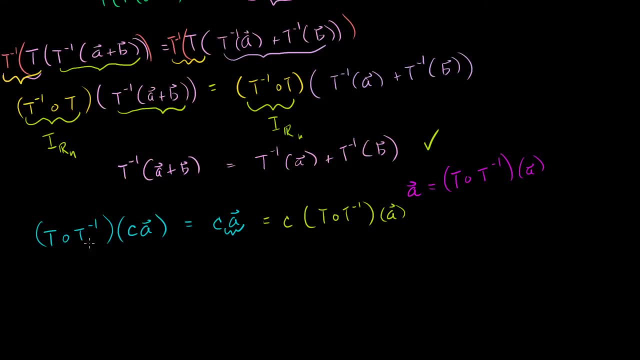 of this composition form. So this left expression. we can just write it as saying t of the t inverse, So t inverse of c times the vector a. All I did is rewrite this left-hand side. this way Is equal to this green thing, right here. 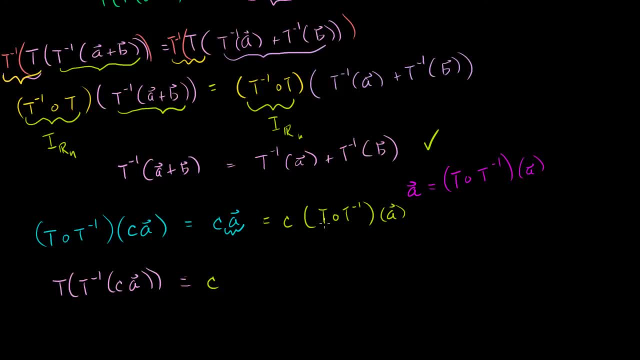 Well, I'll rewrite similarly. This is equal to c times t. the transformation t applied to the transformation t, inverse applied to a. This is, by definition, what composition means. This is what composition means Now. t is a linear transformation. t is a linear transformation. 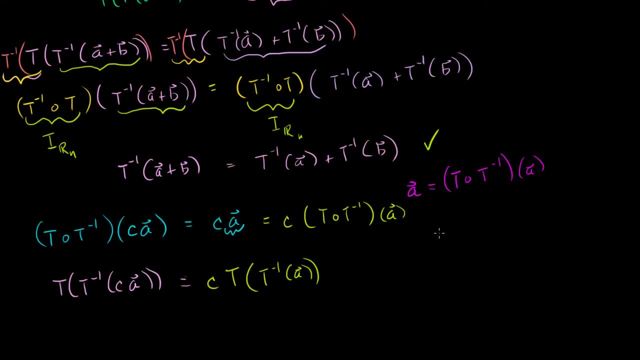 Which means that if you take c times, t times some vector that is equivalent to t, applied to c times that vector. This is one of the conditions of a linear transformation, So this is always going to be the case with t. So this is some vector that t is applying to. 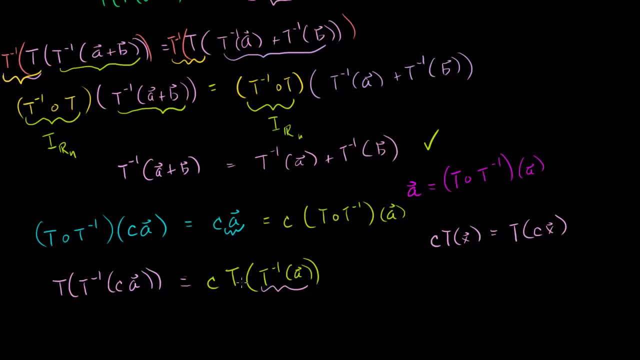 This is some scalar. So this thing, because we know that t is a linear transformation, we can rewrite as being equal to t applied to the scalar c. So t times t inverse applied to a. And now what can we do? Well, let's apply the t inverse transformation to both sides of this. 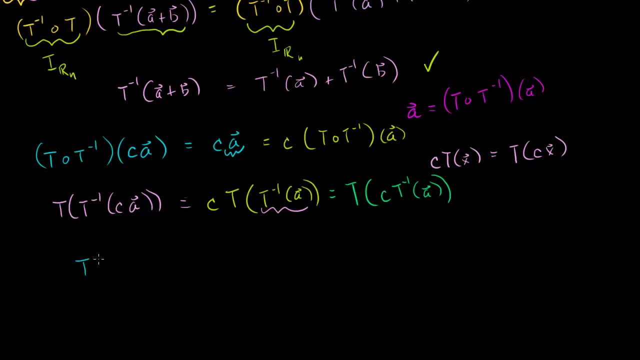 Let me rewrite it So on this side we get t of t inverse of c. a is equal to t of c times t inverse times a. That's what we have so far. Now, wouldn't it be nice if we could get rid of these outer t's? 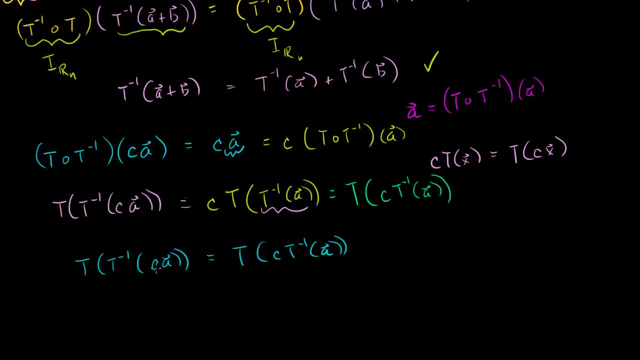 And the best way to do that is to take the t inverse transformation of both sides. So let's do that t inverse, Let's take that of both sides of this equation, t inverse of both sides. And another way that this could be written: this is equivalent. 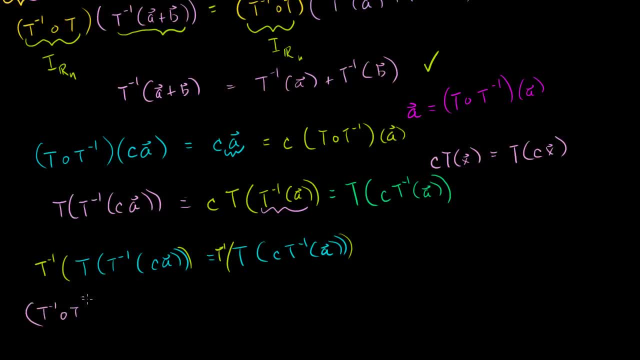 to the composition of t inverse with t applied to c times our vector a. This right here. I've just decided to keep writing it in this form And I took these two guys out and I wrote them as a composition And this on the right-hand side you can do. 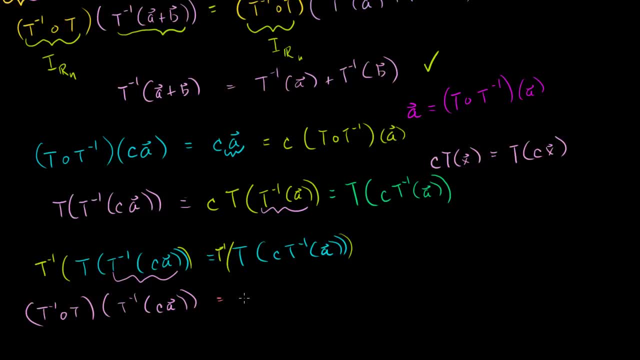 something very similar. You could say that this is equal to the composition of t inverse with t times or not times. let me be very careful: taking this composition, this transformation, and then taking that transformation on c times, the inverse transformation applied to a. 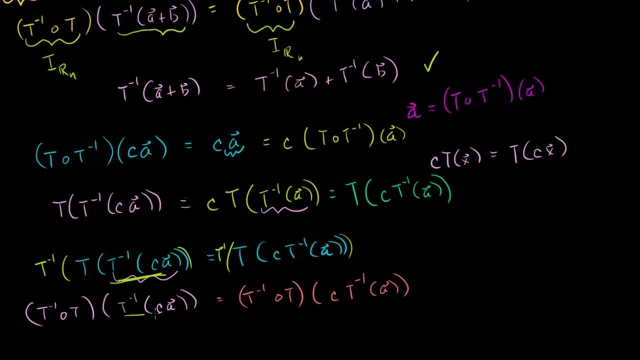 Let me be very clear what I did. This thing right here is this thing right here. This thing right here is this thing right here, And I just rewrote this composition this way. I rewrote this composition this way, And the reason why I did this is because we know that this is. 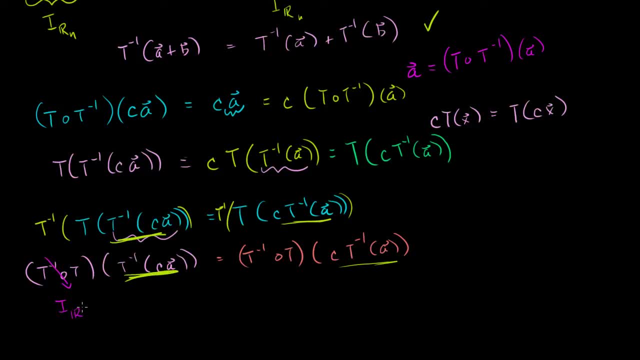 just the identity transformation on Rn. and this is just the identity transformation on Rn. So the identity transformation applied to anything is just that anything. So this equation simplifies to the t inverse. applied to c times, c times, some vector a is equal to this thing: c times t. 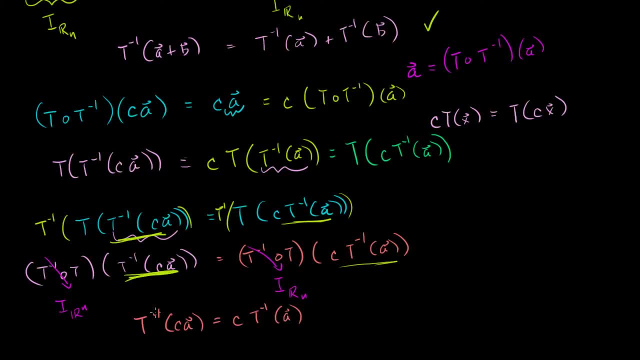 inverse times, some vector a, And just like that we've met our second condition for being a linear transformation. The first condition was met up here. So now we know, And in both cases we use the fact that t was a linear transformation to get to the result for t inverse. 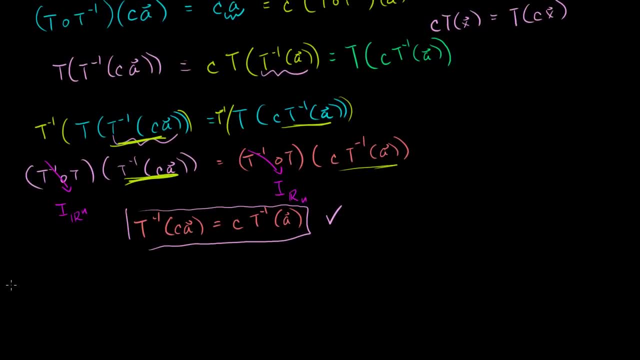 So now we know that if t is a linear transformation and t is invertible, then t inverse is also a linear transformation, Which might seem like a little nice thing to know, but that's actually a big thing to know, because now we know that. 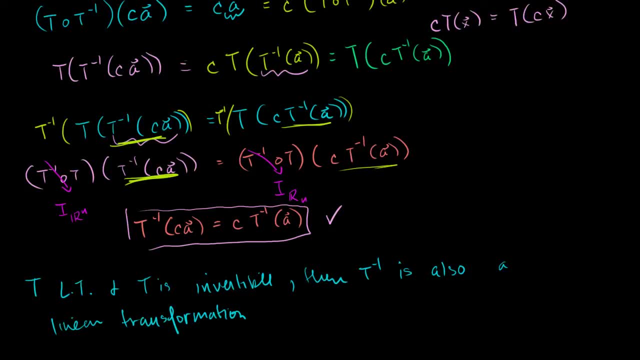 t is a linear transformation. t inverse can be represented as a matrix vector product. So that means that t inverse, applied to some vector x, could be represented as the product of some matrix times x. And what we're going to do is we're going to call that. 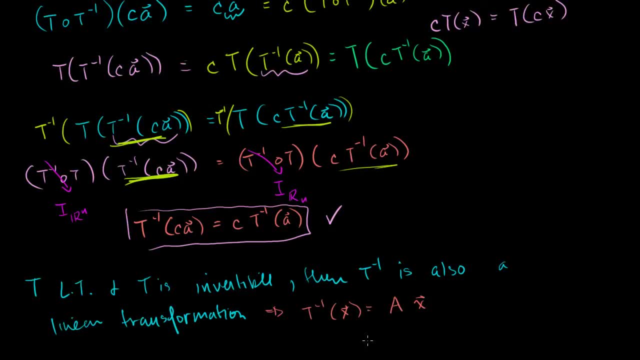 matrix. the matrix A inverse, And I haven't defined this well. How do you construct this A inverse matrix? But we know that it exists. We know that this exists now because t is a linear transformation, And we could take it even a step further. 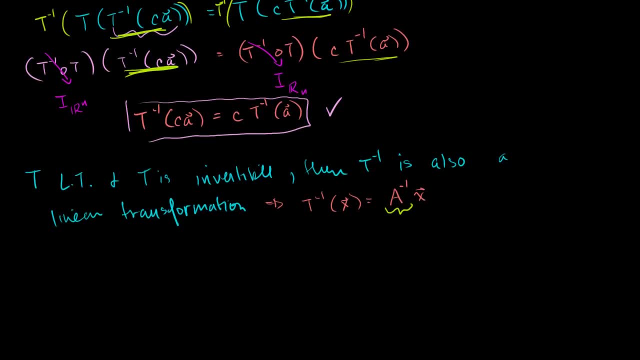 We know, by the definition of invertibility, that the composition of t inverse with t is equal to the identity transformation on Rn. Well, what is the composition? We know that t. if we take, let me put it this way, We know that t of x is equal to Ax. 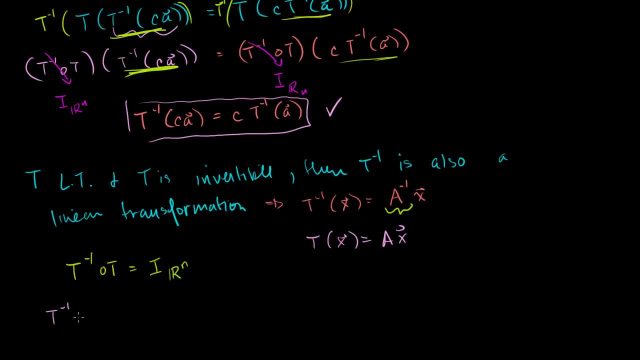 So if we write t inverse, the composition of t inverse, with t applied to some vector, x is going to be equal to first Ax. A being applied to x is going to be equal to Ax- this A right here Ax, and then you're going to apply A inverse x. 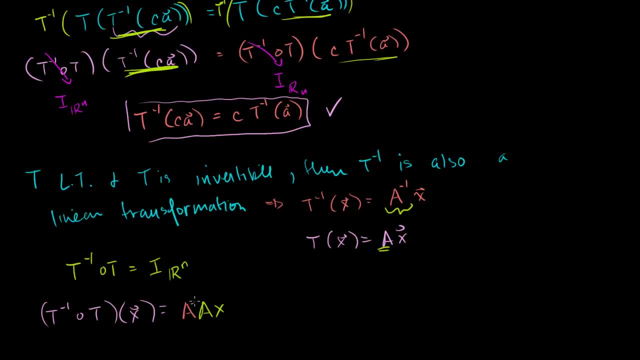 You're going to apply this right here And we got this- that this is equivalent to. when you take the composition, it's equivalent to, or the resulting transformation matrix of two composition transformations is equal to this matrix-matrix product. We got that a long time ago. 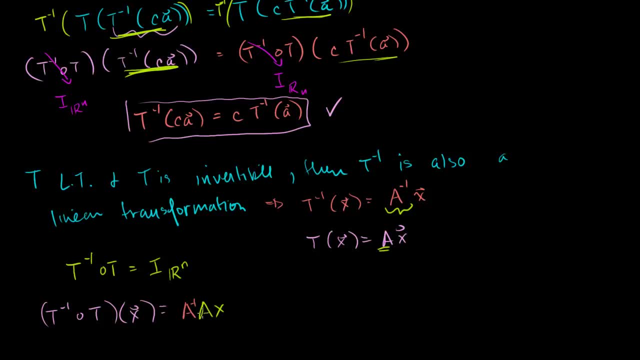 In fact, that was the motivation for how a matrix- matrix product was defined. But what's interesting here is this composition is equal to that, but it's also going to be equal to the identity transformation on Rn applied to that vector x, which is equal. 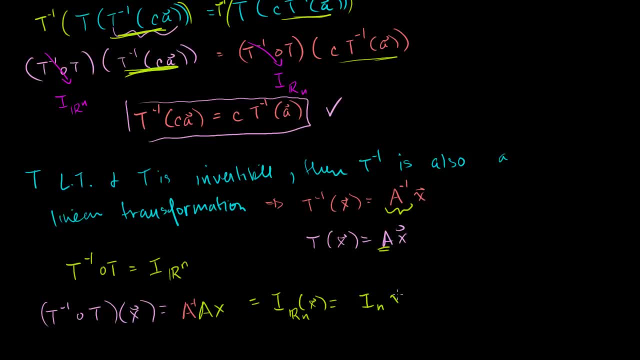 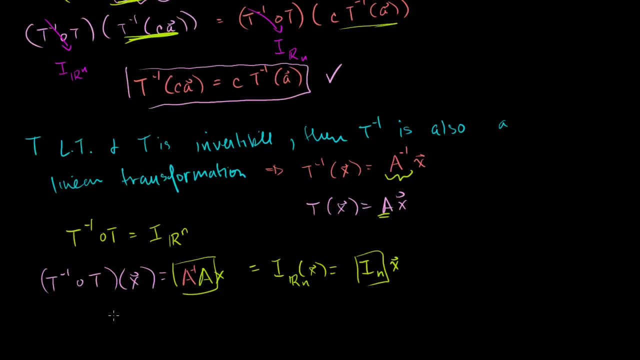 to the identity matrix applied to x Right. That is the n by n matrix Right. So when you multiply it by anything, you get that anything again. So we get a very interesting result. A inverse times A has to be equal to the identity matrix. 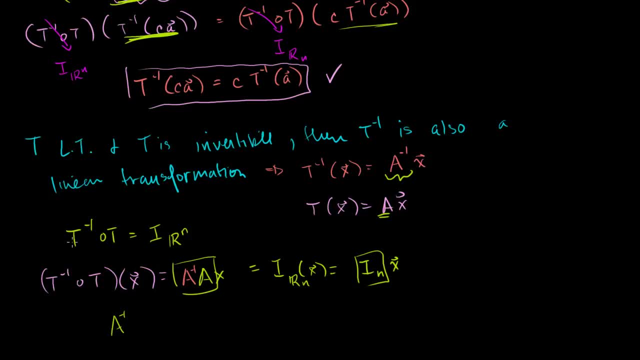 A inverse or the matrix transformation for t inverse. when you multiply that with the matrix transformation for t you are going to get the identity matrix And the argument actually holds both ways. So we know this is true. but the other definition of